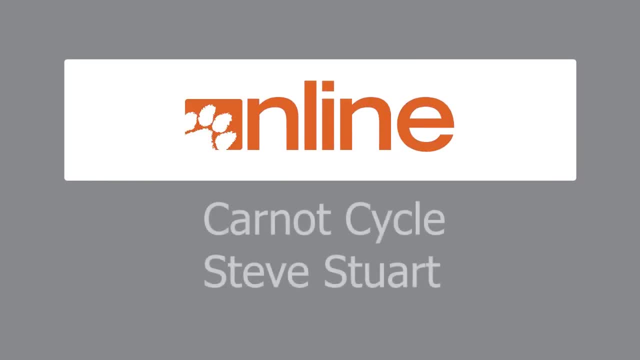 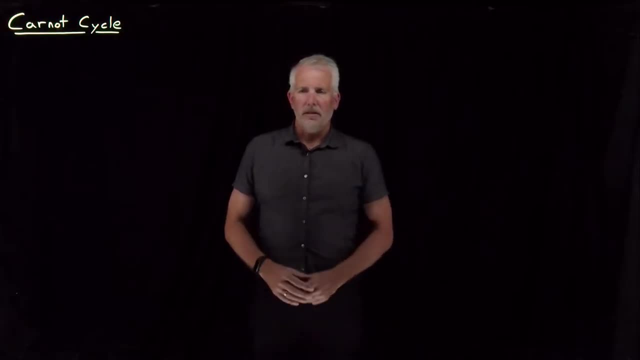 All right, so we understand a fair amount at this point about gases, their PV behavior, how they work when they get compressed or they expand, In particular ideal gases. we've seen equations that describe their PV behavior when we compress them reversibly and isothermally. 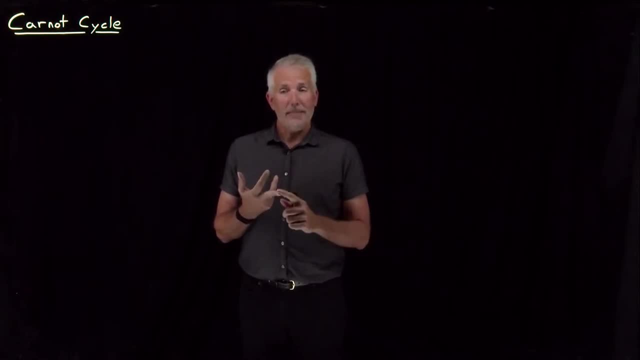 or when we compress them reversibly and adiabatically, two different types of compression. So our next step is to combine those two things, talk about both those types of compression and expansion at the same time, and it turns out we'll discover something fairly remarkable. 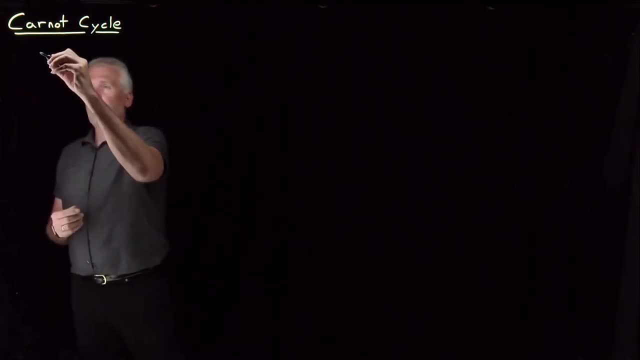 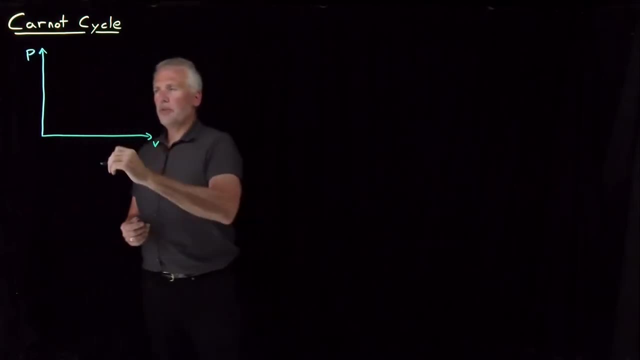 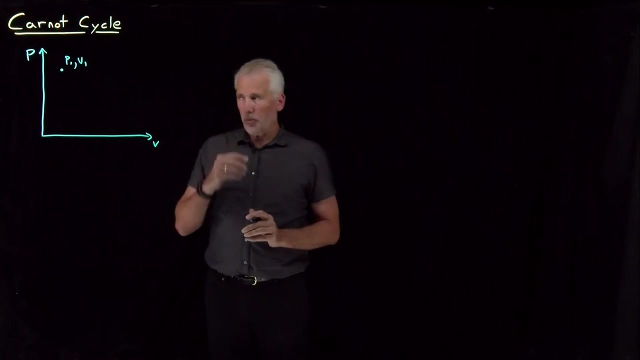 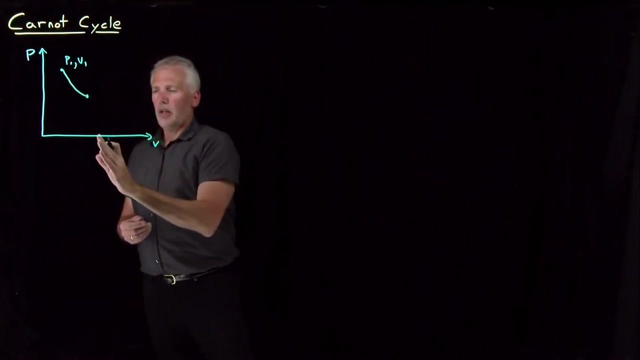 when we do both of those things. So let's start with a diagram, Pressure-volume diagram. We'll start with a gas that's, at some initial pressure, P1, V1. And what I'm going to do is I'm going to compress that gas reversibly and isothermally down to some. no, I'm sorry. 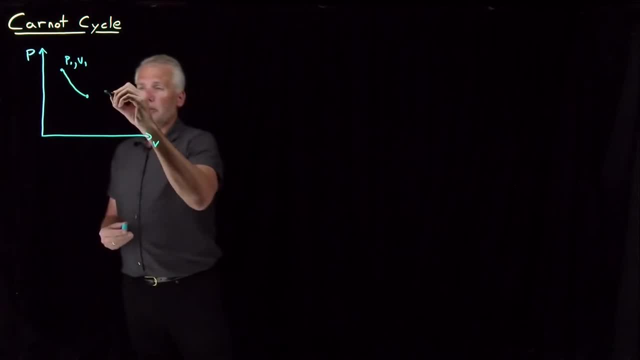 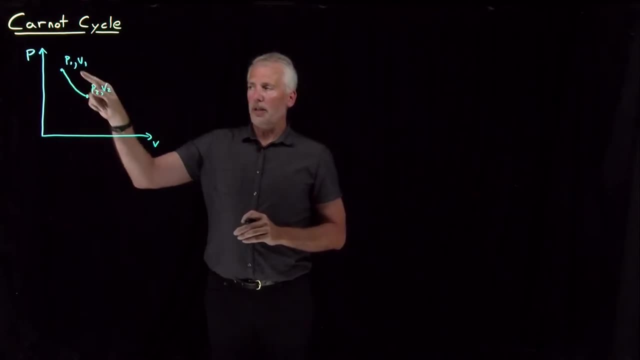 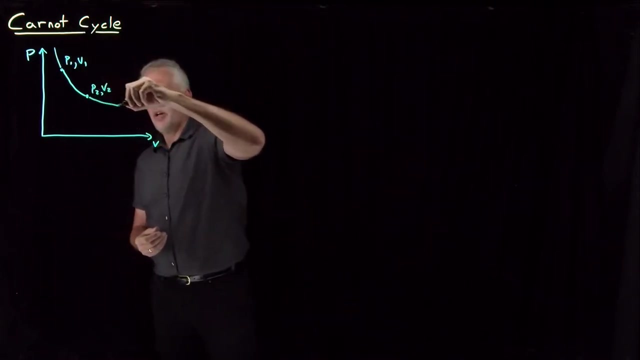 expand. let the gas expand to a higher volume. V2 is larger than V1. So larger volume. so it expands to this larger volume and it's at a lower pressure. I'm doing that reversibly and isothermally. So there's an isotherm here. All the points on that curve are at the same temperature. 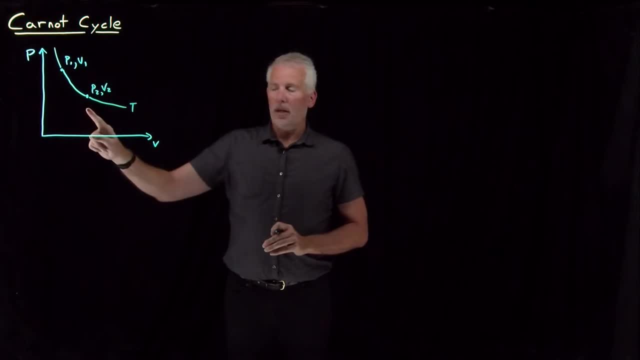 So that's an isotherm. I'm just moving from one point on this isotherm to a different point at that isotherm. So that's the first step in what's going to be a multiple step process. So let me get a little more specific about what's going on in that step. So in 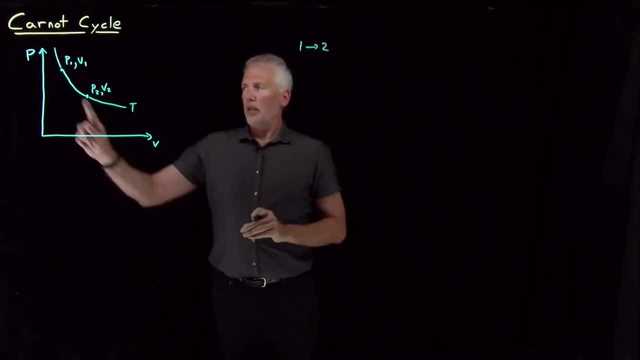 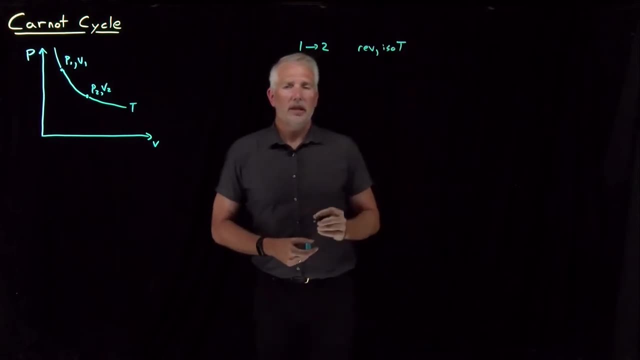 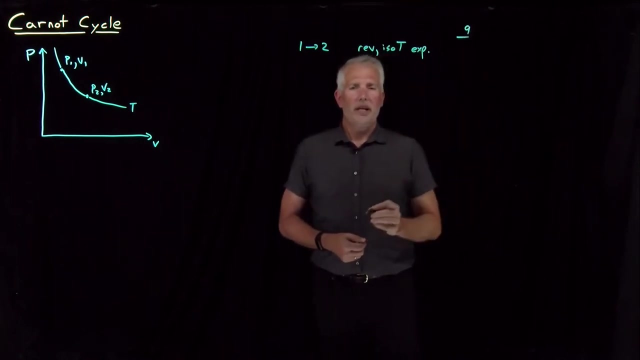 this step, when we go from P1, V1 to P2 and V2, that's going to be our reversible isothermal expansion And we can say how much heat is involved in that process, how much work is involved in that process, how much internal energy change is involved in that process. 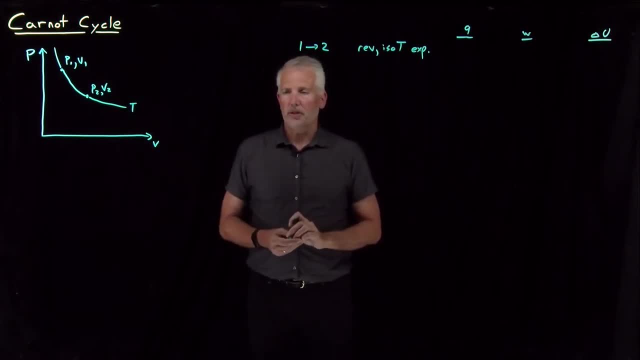 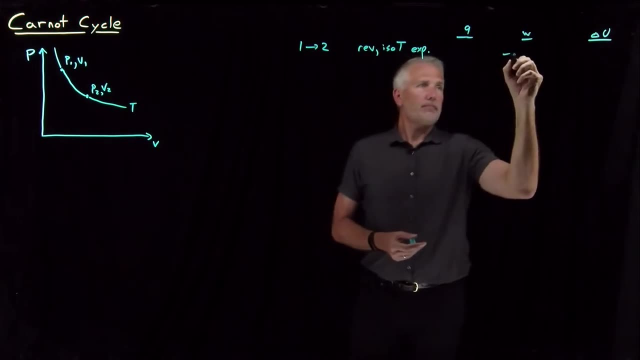 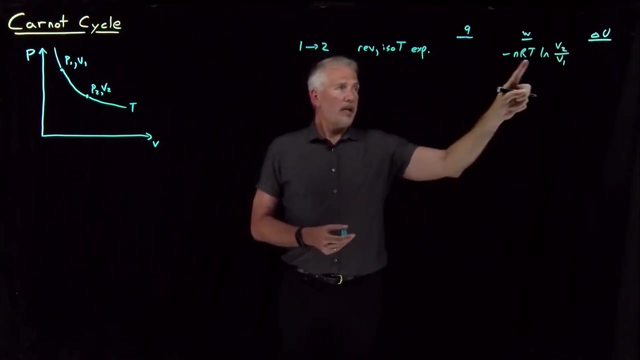 And because we have thought about reversible isothermal expansions already for an ideal gas, we can write down what those are. So reversible isothermal expansions, The work associated with that process is minus nRT. log of V final over V initial. So in this: 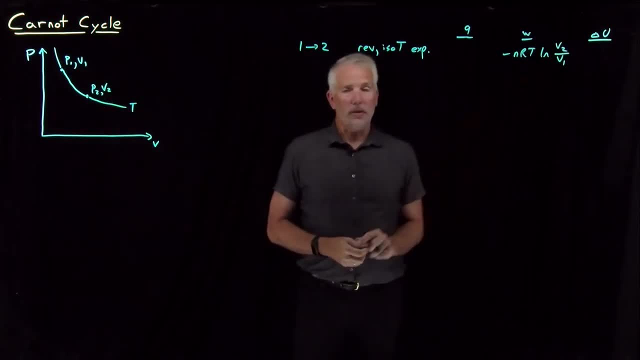 case that's V2 divided by V1. inside of this logarithm It's an isothermal process. So for an ideal gas, delta U is zero whenever the temperature doesn't change. So I know delta U is zero. The work is this. So the heat has to be the opposite of this. So that's. 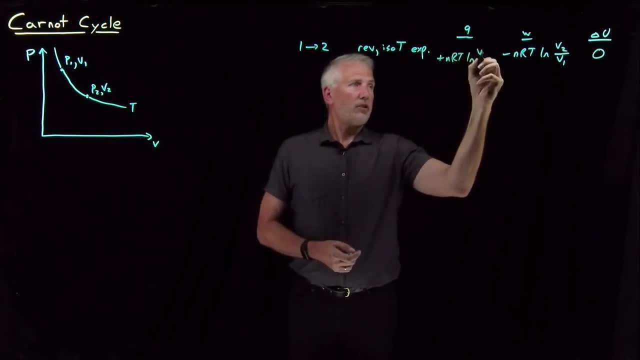 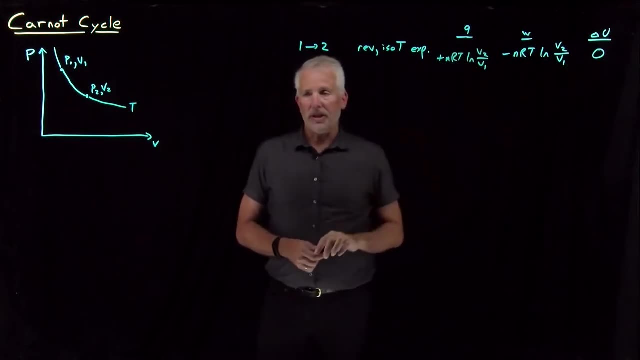 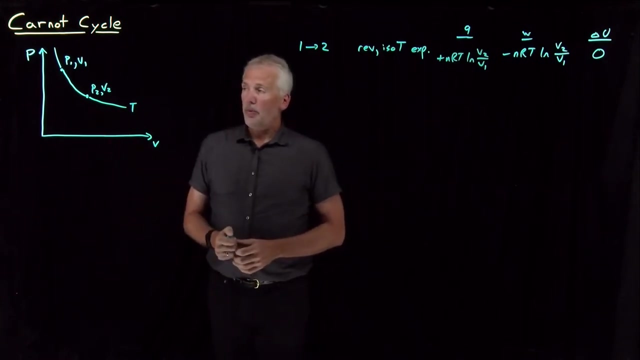 going to be positive nRT natural log of V2 over V1.. All right, So that's just repeating what we know about work heat and internal energy change for reversible isothermal expansion of an ideal gas. Next, what we're going to. 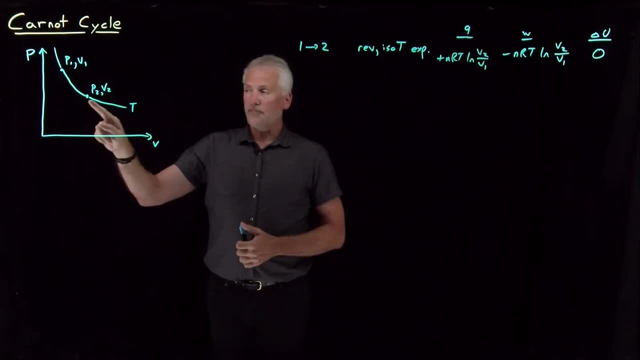 do is, after we've expanded the gas to P2 and V2, still on this isotherm- we're going to expand it a little more. But now, instead of expanding isothermally, instead of remaining on this isotherm, we're going to expand adiabatically. So I'll draw that curve in a different color. 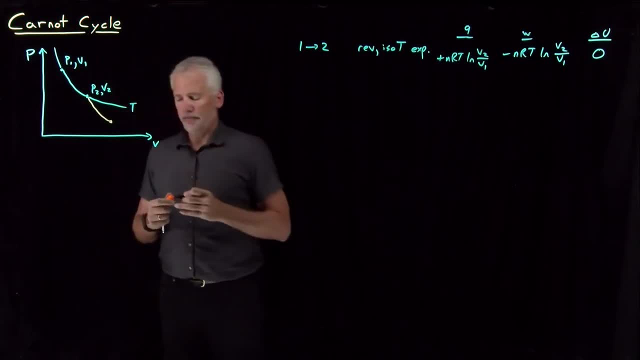 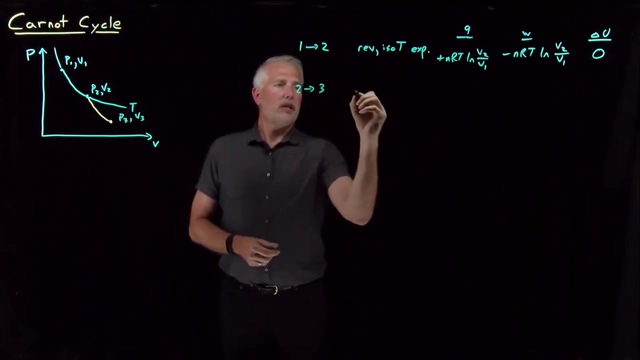 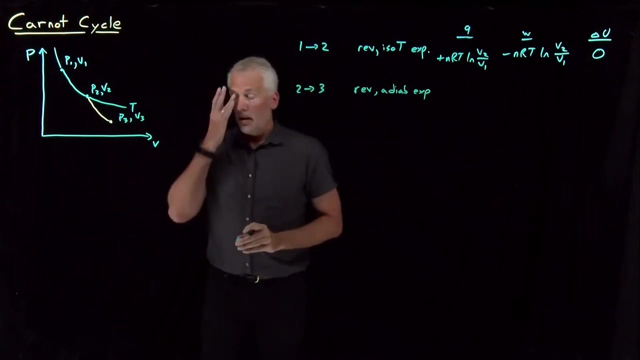 And that curve is going to look something like this because it's going to expand to some new P3 V3. When I go from step two to step three, that's going to be a reversible and adiabatic expansion. I know to draw the curve in this way because, as we know from 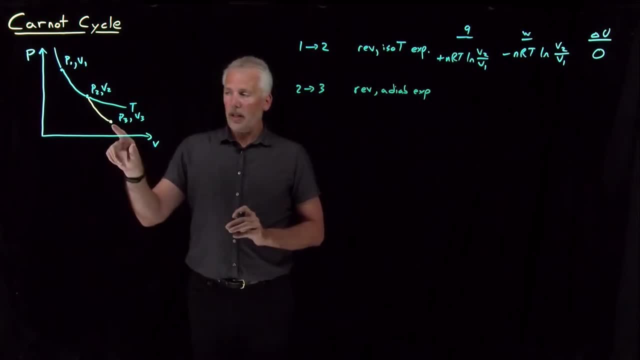 talking about adiabatic expansion. I know to draw the curve in this way because, as we know from talking about adiabatic expansion, P3 changes. when a gas expands adiabatically, its temperature drops, So it's no longer on. 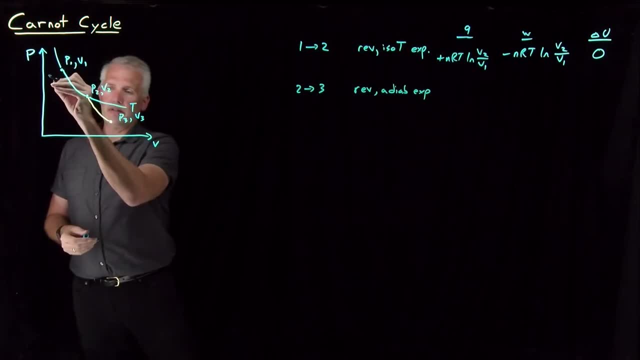 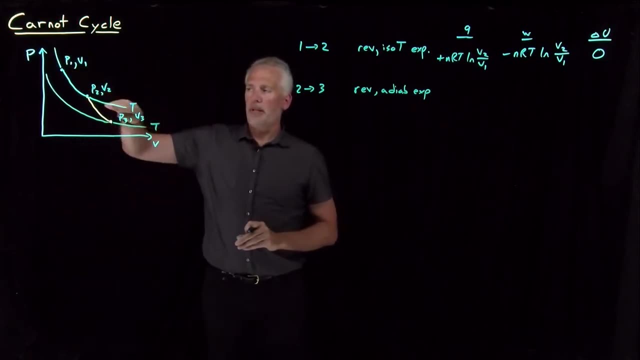 the same isotherm There's a different isotherm that it lives on. So here's a set of P V conditions that are all at the same temperature for the gas. Here's another set of P V conditions that are a different temperature. So the first curve I'll say that's T hot, TH for T hot. 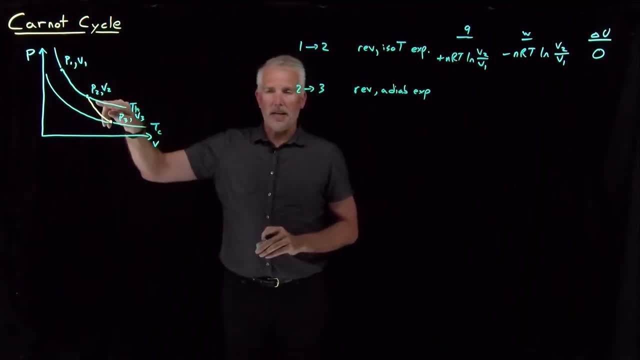 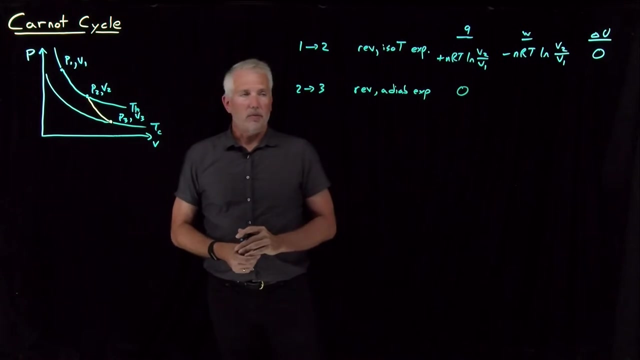 This one is TC for T-cold. The upper isotherm is at a hotter temperature than the lower isotherm, So I've done this adiabatic expansion down to a colder temperature. What we know about adiabatic expansions? first of all, it's adiabatic and reversible, so the heat is zero. 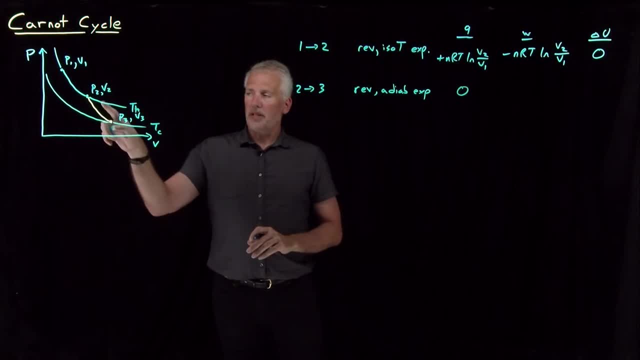 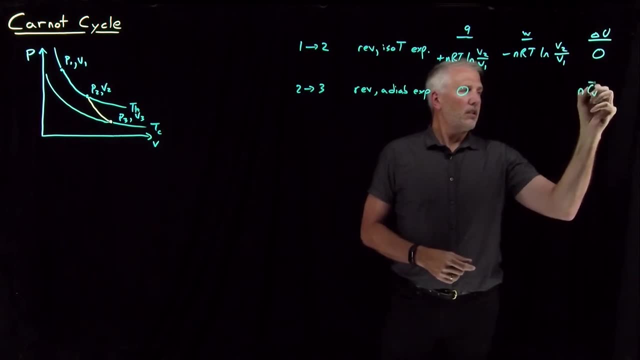 Secondly, probably the easiest way to think about this is: the temperature has dropped for an ideal gas. If the temperature changes, the change in the internal energy is going to be moles times the molar heat capacity, times the change in temperature. In fact, let me not say CV, because we're not at constant volume. 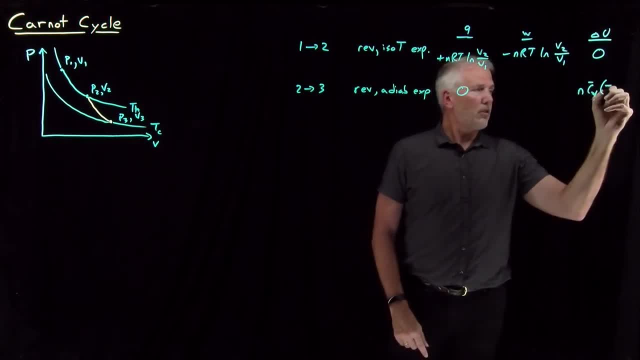 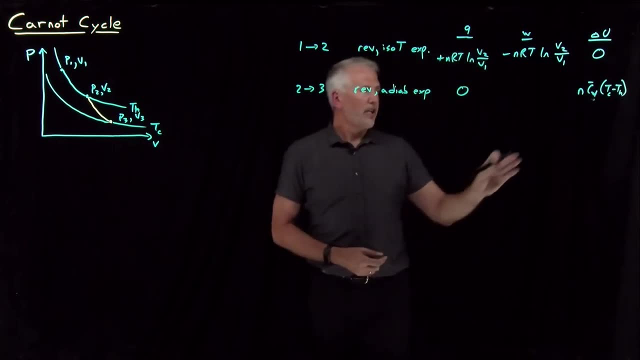 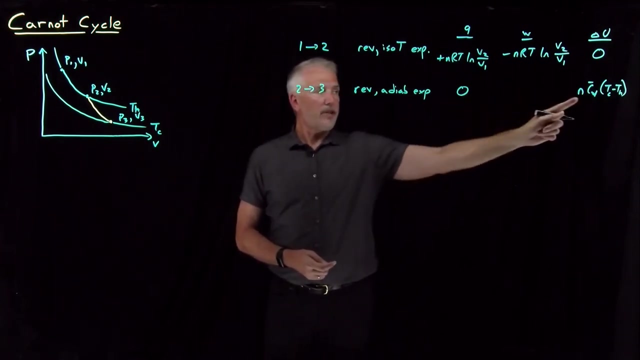 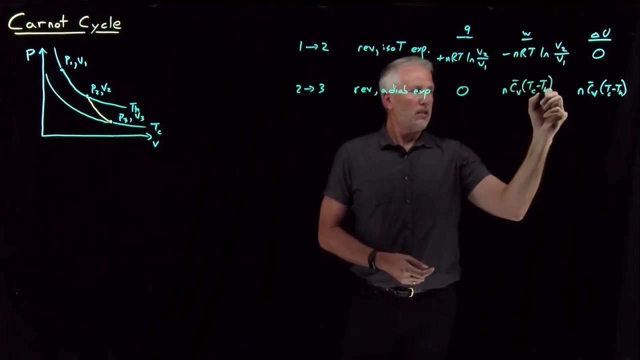 Yes, yes, I do want to say CV. So final temperature T-cold, minus. initial temperature T-hot. The change in the internal energy is NCV times this change in temperature. And again, because heat and work have to add up to the internal energy, the work must also be the same value. 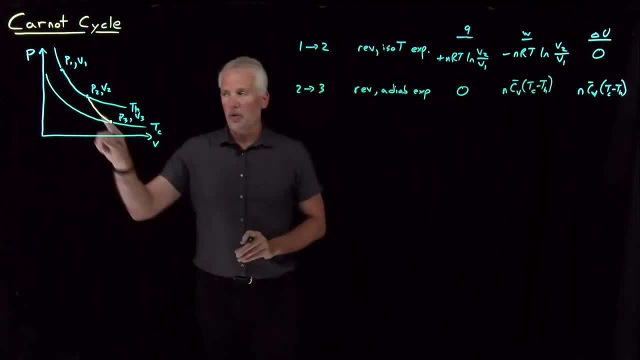 So those are the heat work and internal energy change. when I do this adiabatic expansion Now, the next step in this process- we're going to eventually get back to where we started. So the next step is to get back to where we started. 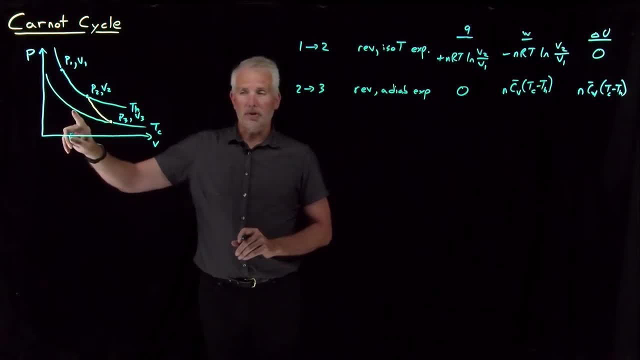 So the next step is to get back to where we started. So the next step in this process is to climb back up this lower temperature isotherm. So now I'm going to do a compression to lower volumes and it's going to be an isothermal compression. 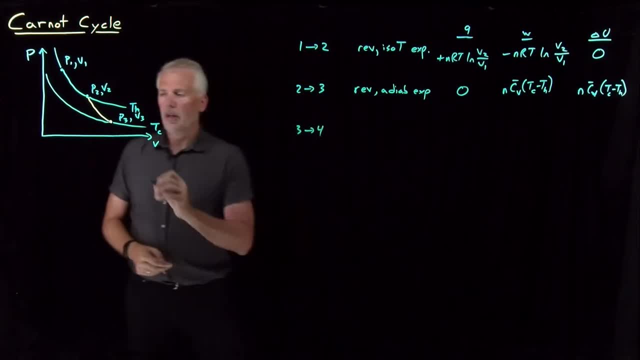 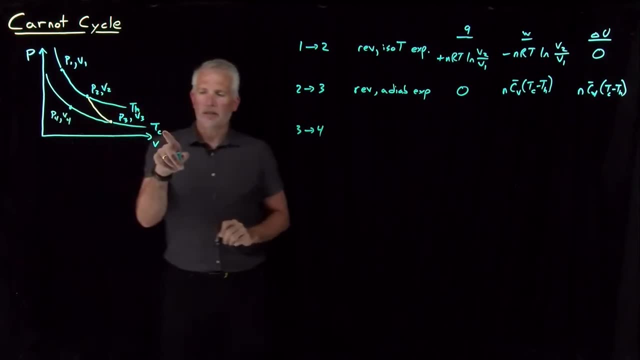 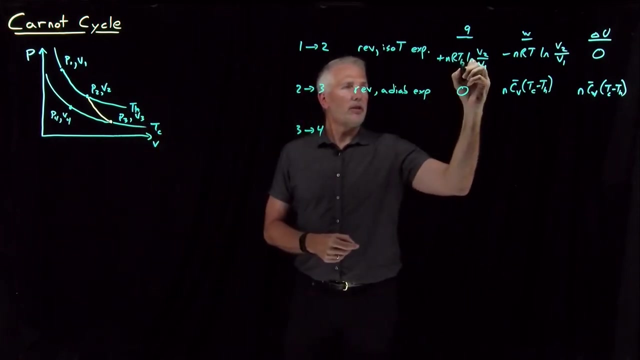 So, step from three to four. I'm going to climb back up the isotherm to some point that I'll call P4V4, that's at this cold temperature. And now that I've labeled these temperatures hot and cold, let me remember that the first isothermal expansion took place at not temperature T-cold. 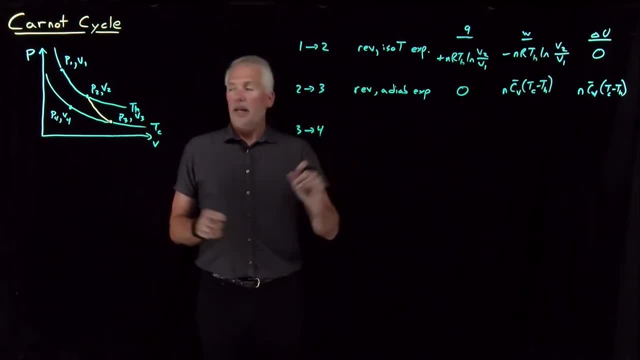 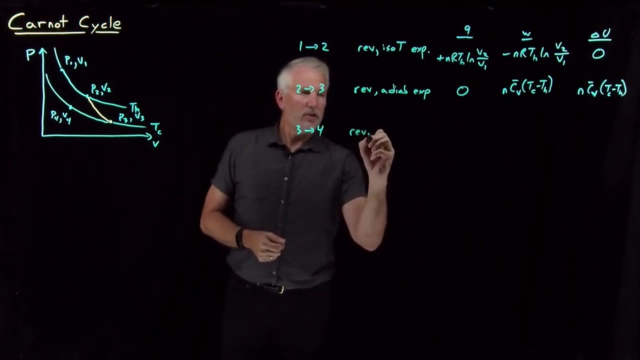 But temperature T-hot. I renamed it, This second isothermal process. the compression is happening at T-cold. So I'm using the same equations for heat work, internal energy of a reversible isothermal process for an ideal gas. This one is a reversible isothermal compression. 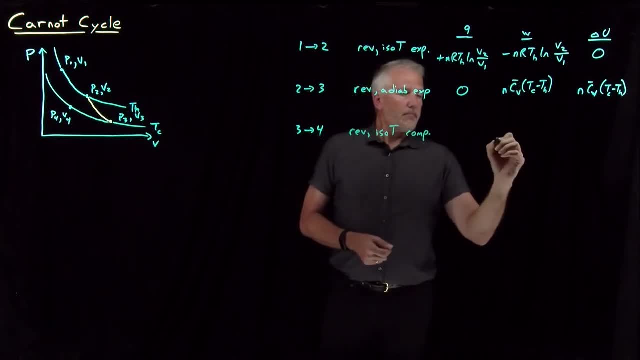 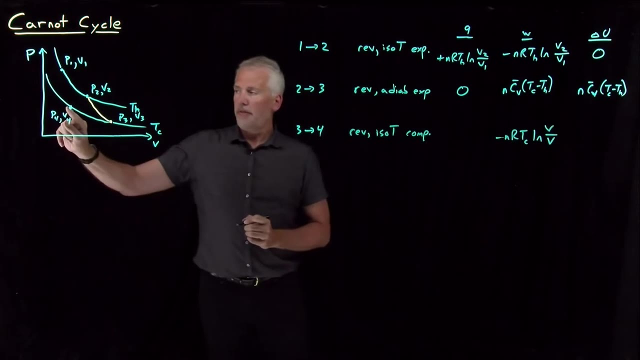 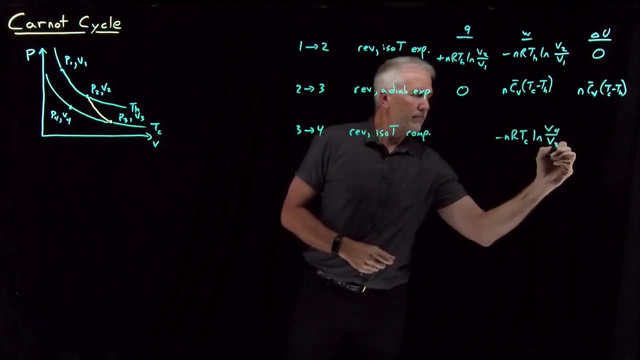 The work is still negative. nRT log: V final over V initial. Let's label these carefully. the temperature at which I'm doing this process is the cold temperature Tc. V final over V initial is V4 over V3, And that's what I've got for my work. 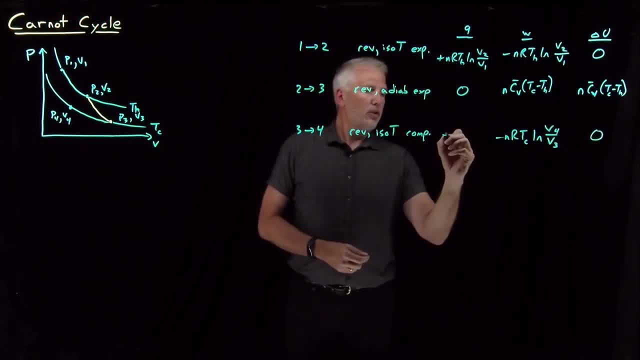 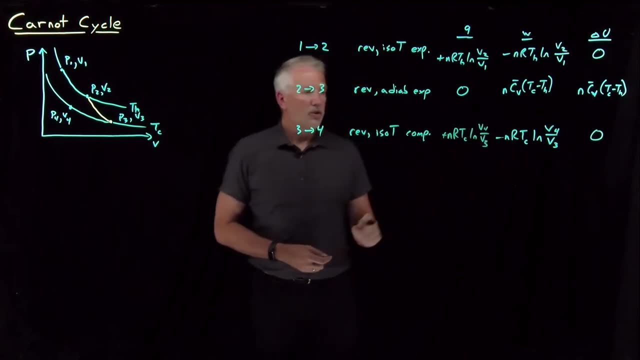 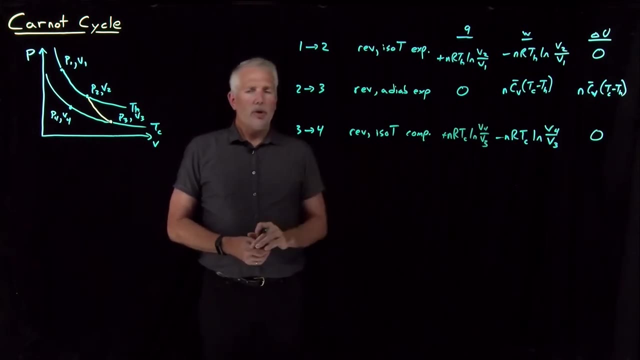 Isothermal, so there's no internal energy change. Q and W have to add up to zero, So heat is positive. nRT cold log of V4 over V3. Before we go any further, I'll point out that we actually know something about this ratio of V4 and V3. 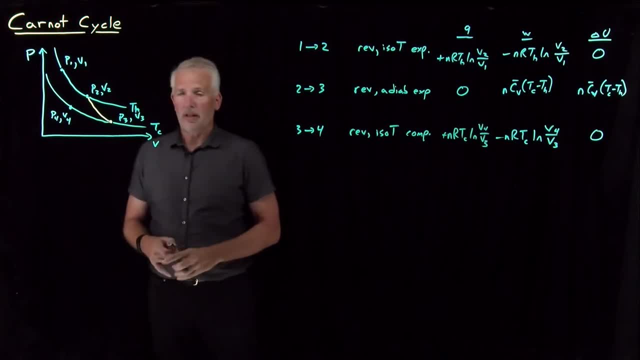 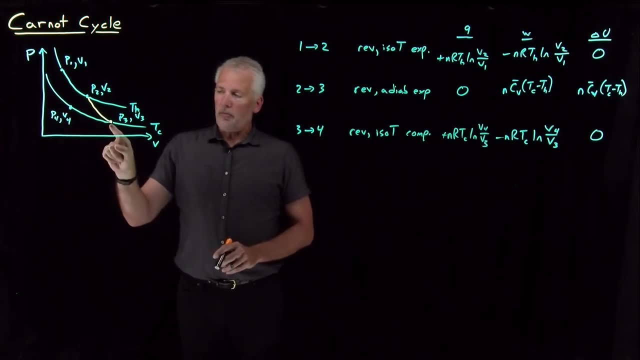 Specifically if I tell you that the next step in the process is going to be another adiabatic expansion up to where I started. so This third step where I go from P3- V3 up to P4- V4- I don't want to stop just anywhere. 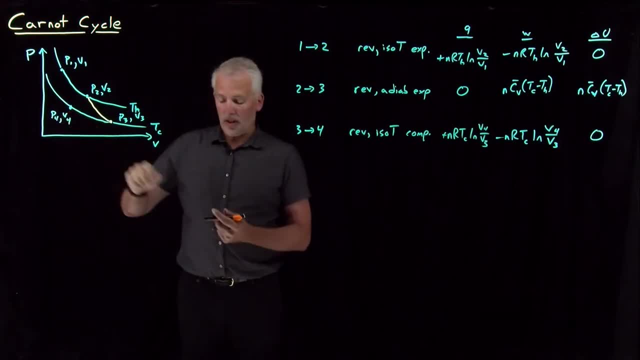 On this isotherm. I want to stop at the specific place where, if I then Adiabatically compress the gas, I'm going to get right back to where I started. So there's a particular point on this curve where an adiabatic compression will lead me back to my initial conditions. 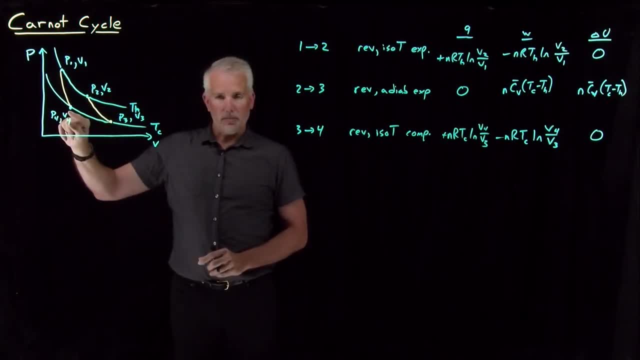 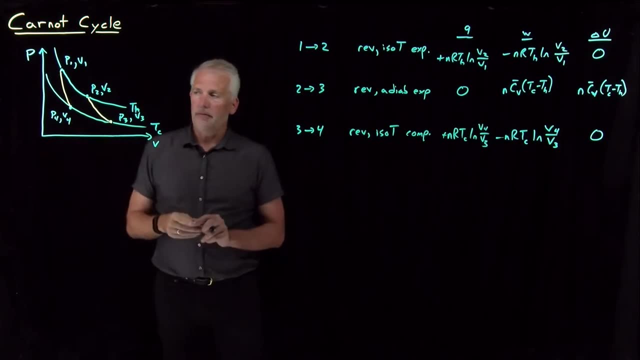 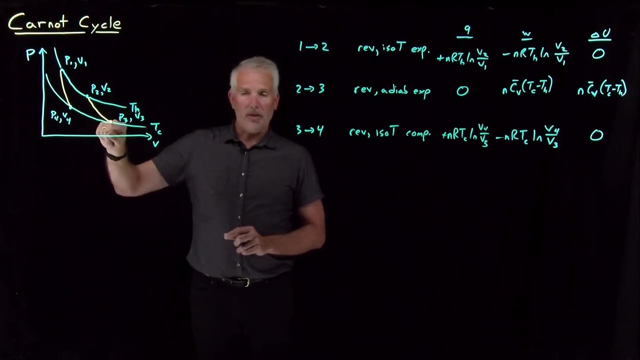 That's exactly where I want to stop this reversible isothermal compression. That particular point. we know something about this V4, in fact, for the adiabatic expansion step, when the gas cooled down during the second step, when I adiabatically Expanded it, we know that. 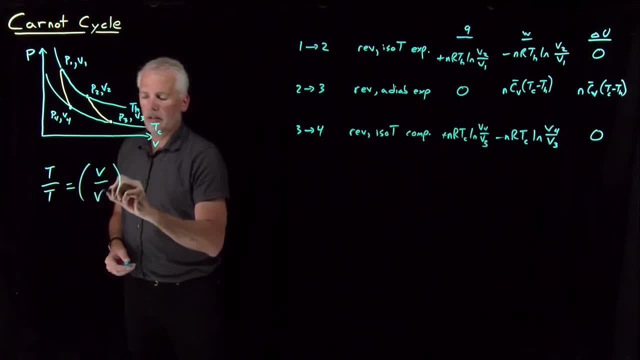 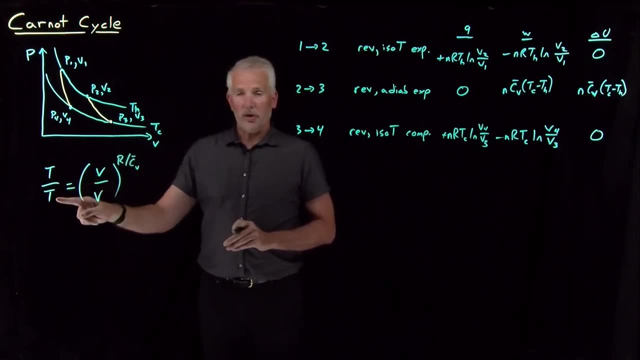 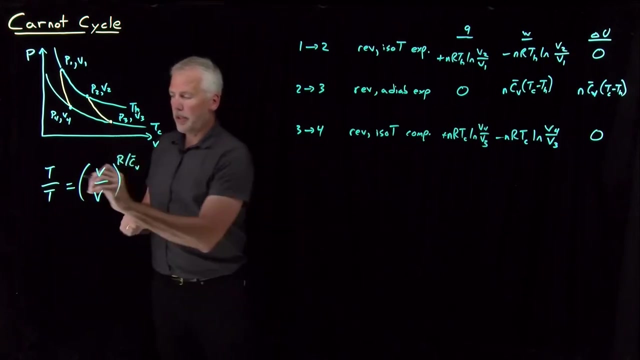 From what we determined When we thought more deeply about adiabatic expansions. the ratio of temperatures T final over T initial is the opposite ratio of the volumes, volume initial over V final. raised to this power, R over C, V bar. so, Labeling my finals and initials carefully, my final temperature in the expansion was the cold temperature, so T cold over T hot is. 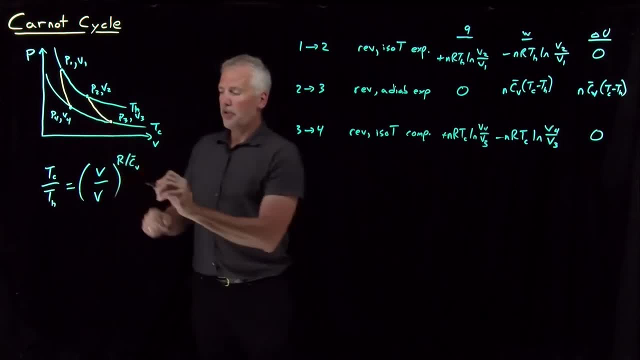 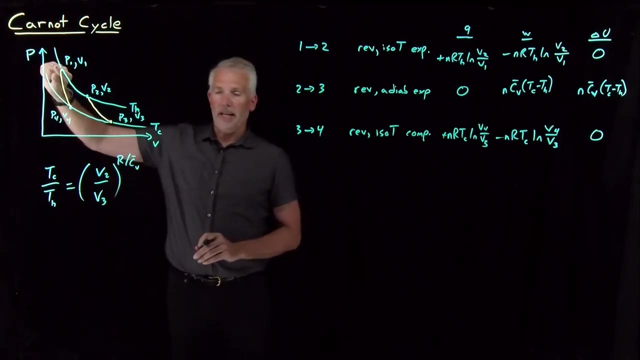 Equal to V initial over V final, so that's V2 over V3 Raised to these powers. That's also the same, The difference in this adiabatic cooling from T hot to T cold. that would have been the same as if I adiabatically cooled from. 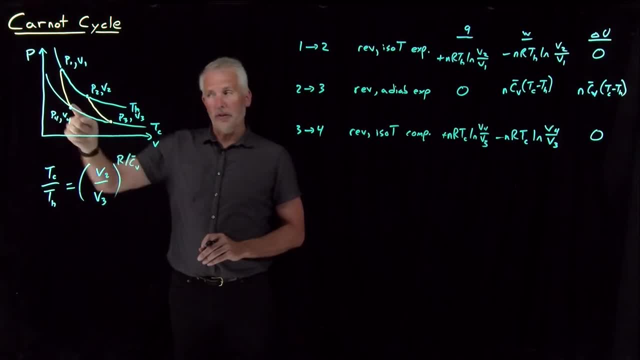 P1 V1 down to this P4 V4, or equivalently if I adiabatically compressed up to the hotter temperature. So this ratio- T cold over T hot- is This ratio of volumes raised to this power. It's also this ratio of volumes. 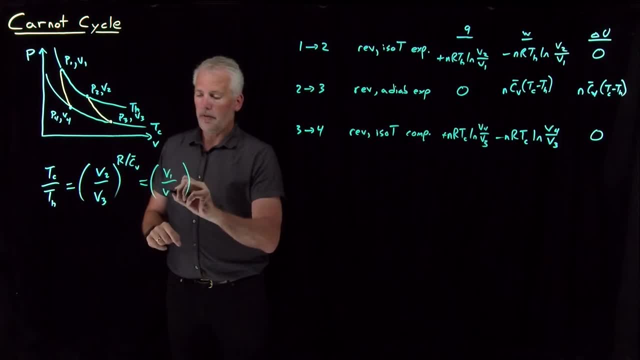 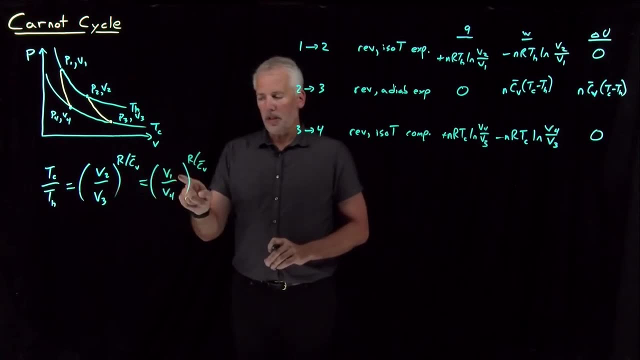 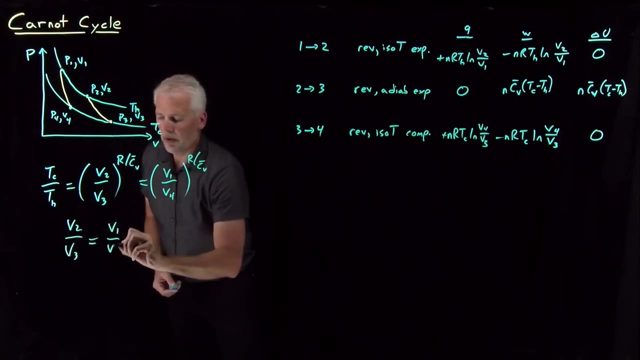 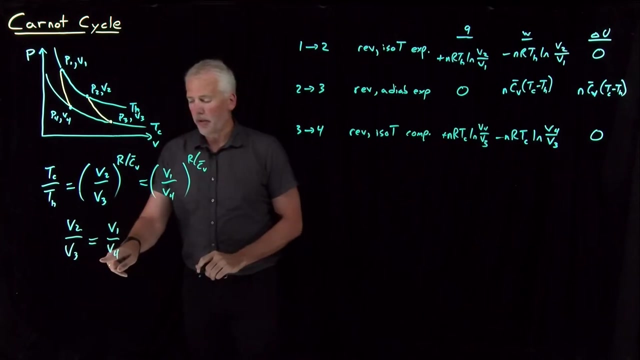 V 1 over V4 raised to the same power. So if this ratio raised to a power is equal to this ratio raised to a power, it must be true that V2 over V3 Is V1 over V4 Or, Since I have this ratio, V4 over V3, if I rearrange this, if I put V4 up here, 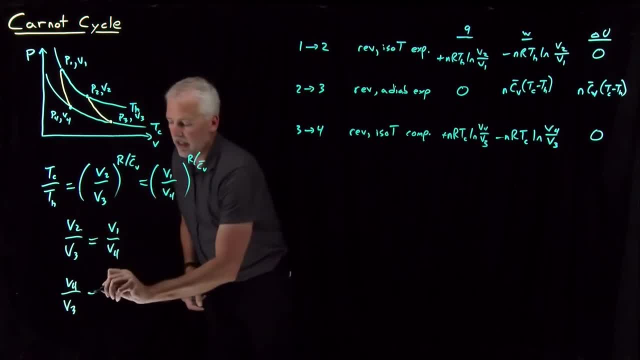 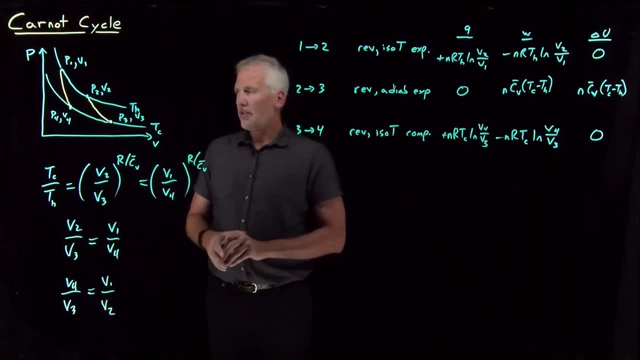 And Therefore I have to take V2 over to the other side. This ratio V4 over V3 is the same as the ratio V1 over V2. Let's make sure we understand what that means. this volume Relative to that volume. so this the value on the V axis relative to this value on the V axis. 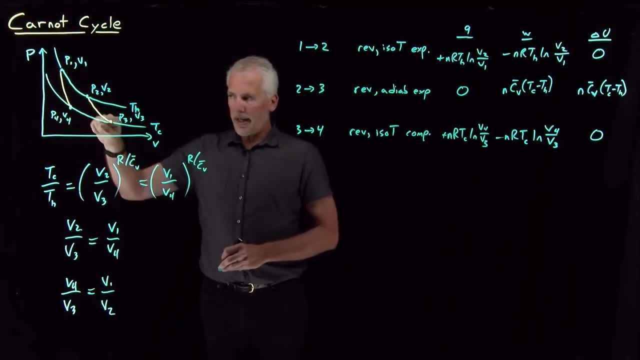 that ratio is exactly the same as this ratio. If this adiabatic expansion doubled the volume, this adiabatic expansion or compression also doubled the volume. So that's perhaps not a surprising fact, but it's one that takes a little bit of thought. 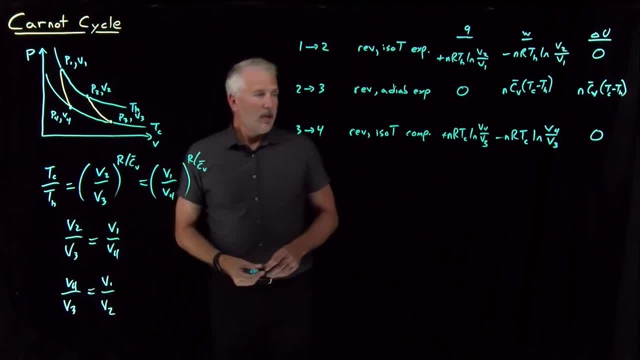 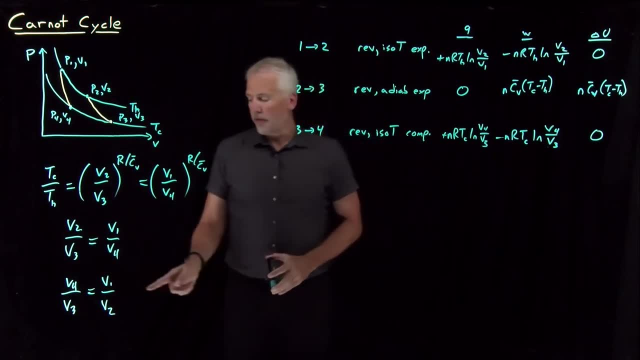 to convince us that we do in fact know that that's true. So when I write minus nRT cold log of V4 over V3, I could equivalently rewrite V1 over V2.. In fact, I'll go ahead and do that. 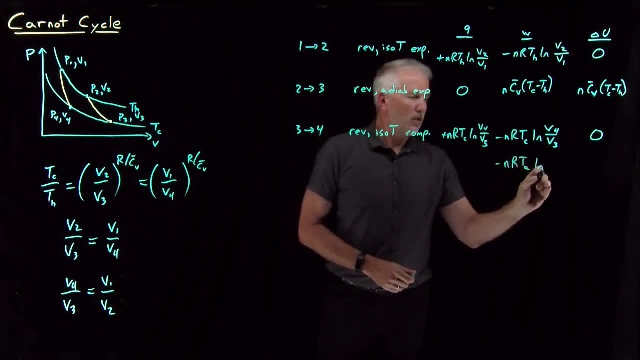 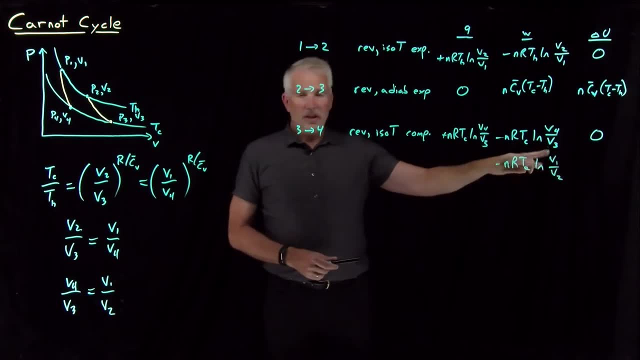 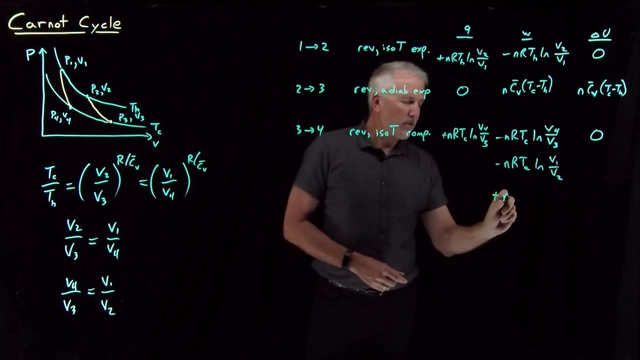 Minus: nRT cold log of V1 over V2.. Or if I wanna exchange the positions of V1 and V2, which I do to make it look more like this one, I can change the sign out front and I'll write that as positive: nRT cold log V2 over V1.. 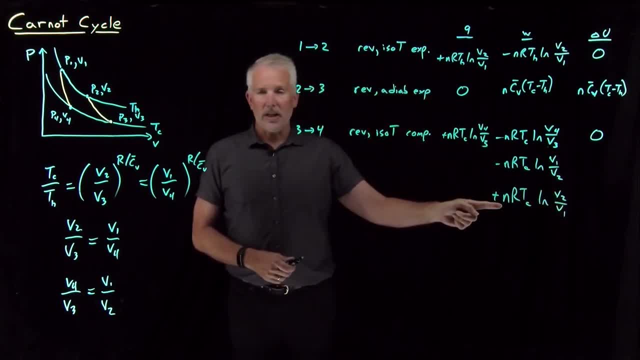 Any one of these three ways of writing, it is exactly the same. I like this last one best because it has a log V2 over V1, which looks a lot like this one Same thing for heat, So nRTC log V4 over V3,. 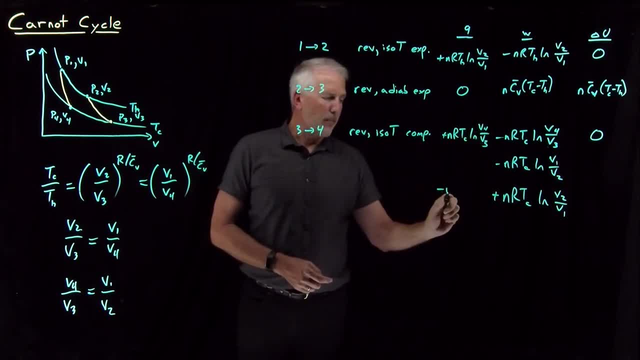 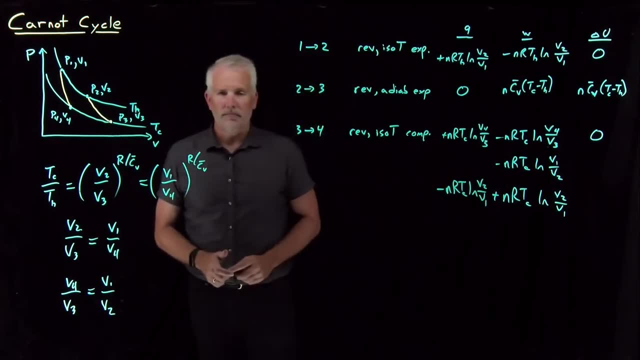 I could write it as V1 over V2, or I could change the sign and write it as minus nRTC log: V2 over V1.. All right, Heat. this column is our work for this third step, the adiabatic compression. 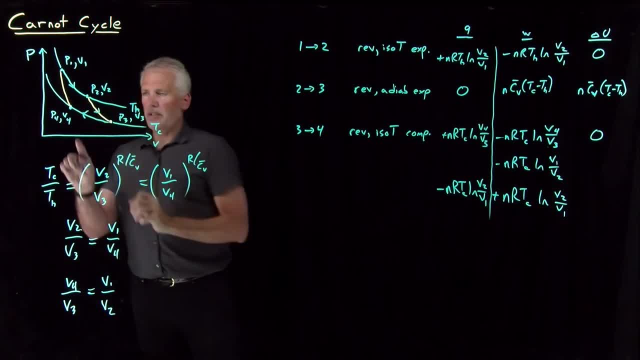 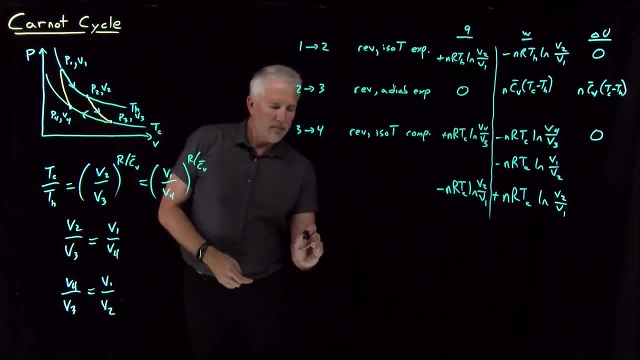 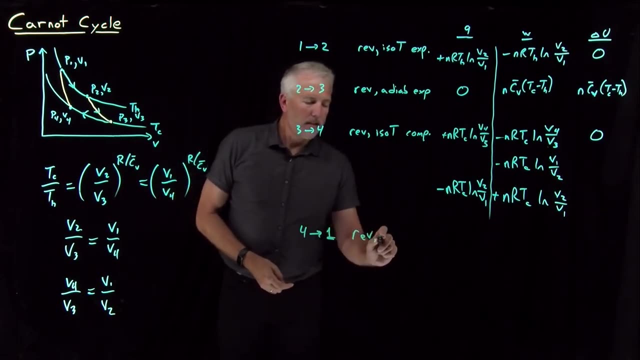 So I've expanded, expanded again, compressed now to P4 and V4.. My last step is to compress the rest of the way from V4 up to V1. So for this step, the step for four going to one that's gonna be another adiabatic. 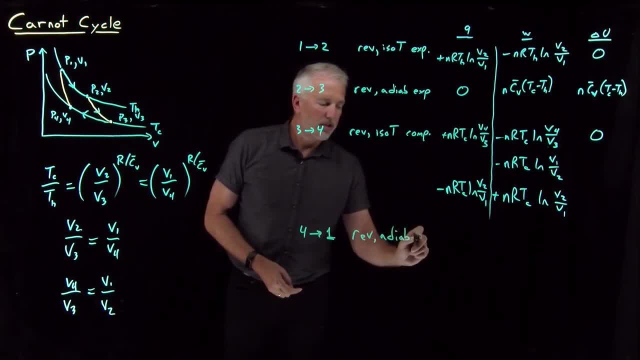 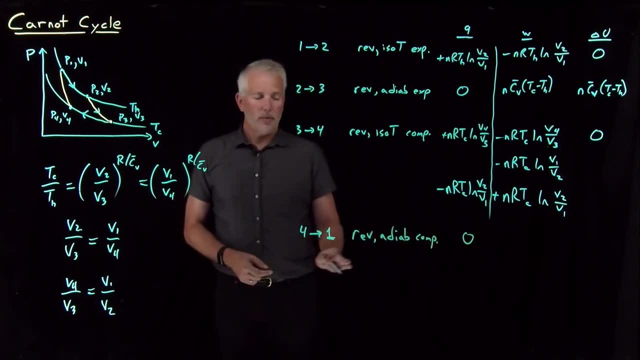 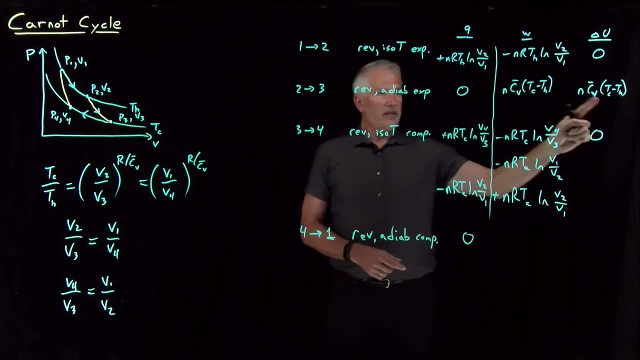 reversible and adiabatic step. This one is a cool one. So the compression, like any adiabatic process, there's no heat associated with it. any reversible adiabatic process, The work and the delta U, as in the adiabatic expansion. 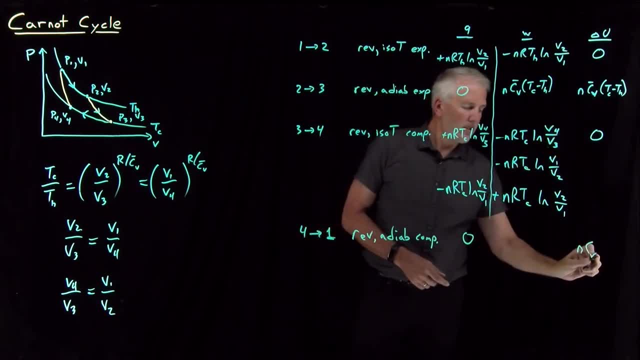 are gonna be the same number. In this case, I've changed. instead of changing from T hot to T cold, I've changed from T cold to T hot, So this is just the same thing in reverse. I've gone. my final temperature is T hot. 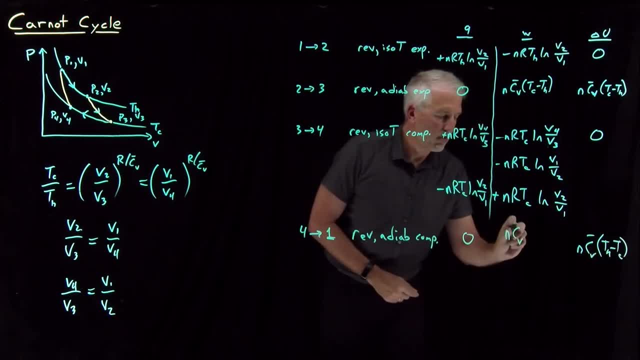 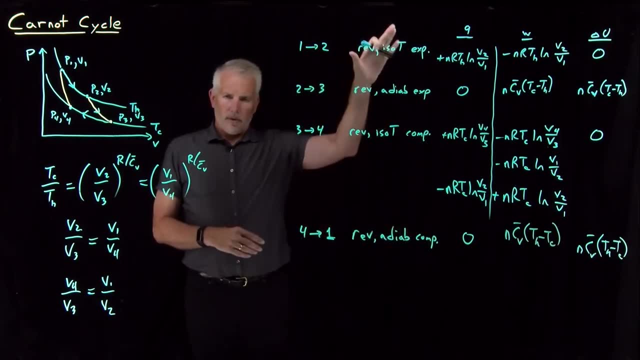 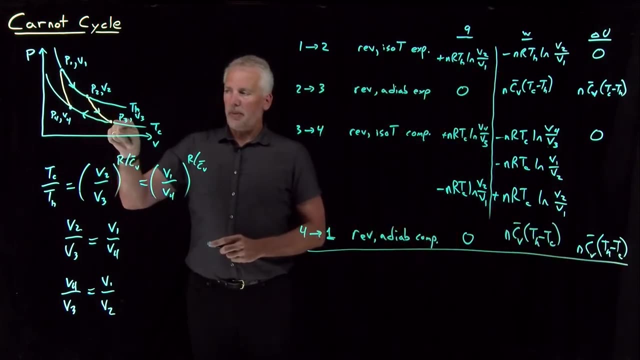 my initial temperature is T cold, T cold. All right, So we're done with our four-stage process. expand, expand, compress, compress. get back to where we started. This is a cycle, a cyclic process, because I ended up back. 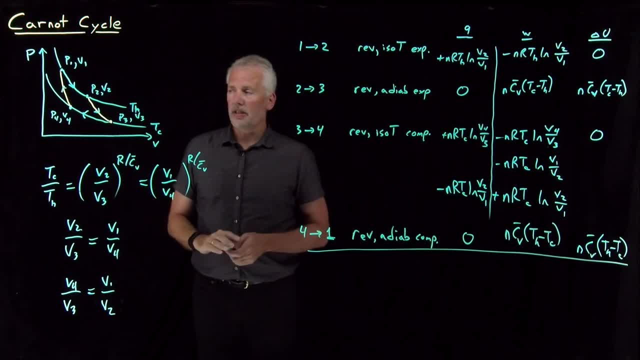 where I started. It's called specifically the Carnot cycle, the sequence of doing a reversible and then adiabatic expansion, followed by a reverse- I'm sorry- isothermal and then adiabatic expansion, followed by isothermal and then adiabatic compression. It's called the Carnot cycle. after, 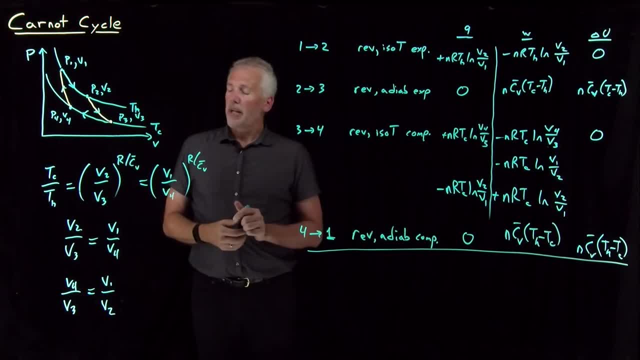 Sadi Carnot, a French thermodynamicist from the 1800s. What's special about this process in particular that we've done for the ideal gas? let's take a look at what all these numbers add up to. So if I do all four steps in sequence, ending back up where I started, the total 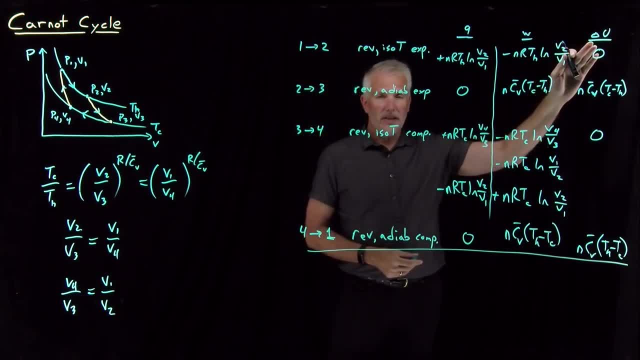 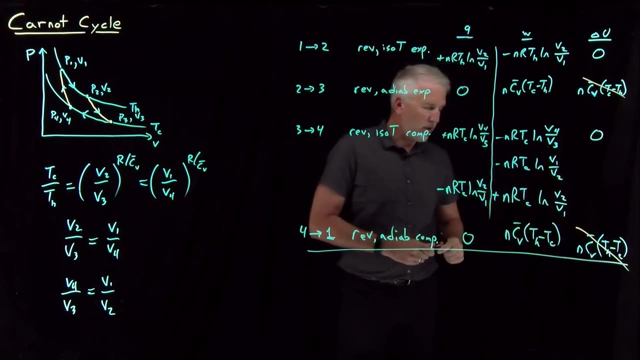 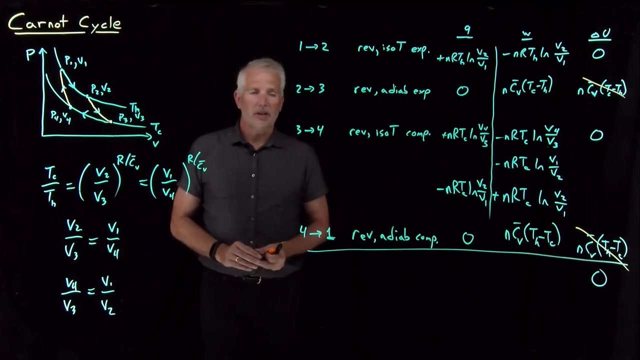 amount of internal energy change. delta U zero and zero. NCV times cold minus hot. If I add that to NCV times hot minus cold, those two terms exactly cancel each other. So the net amount of internal energy change for the process is zero. That shouldn't be too surprising, because internal 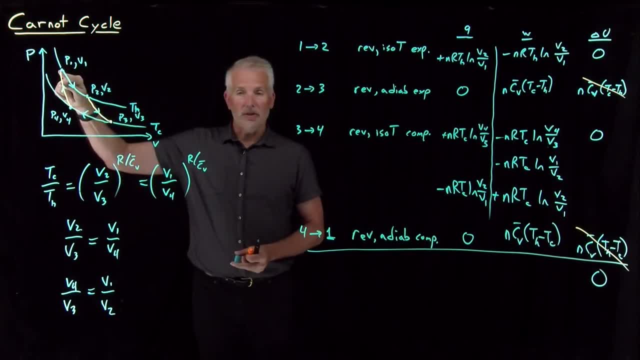 energy is a state function. Whatever I do, if I end up back where I started, the internal energy at that state is exactly the same. So if I go away and come back, the change in the internal energy has been zero. Heat and work, of course, are not state functions. So if I add these up, I 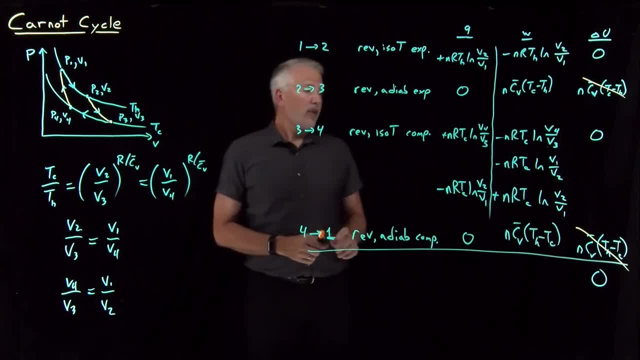 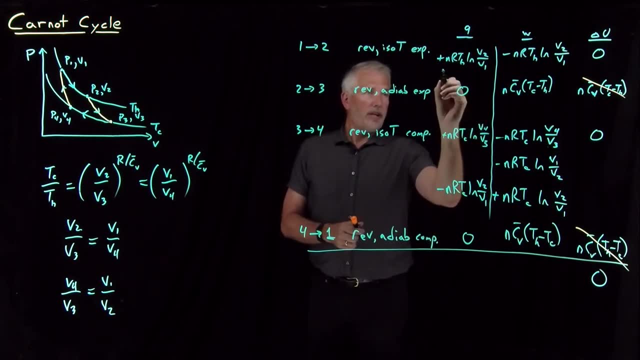 won't get zero. I won't necessarily get zero, and I don't get zero In this case. let's see if I add up some zeros, if I add up this term and this term for the heat. remember, this is just another way. 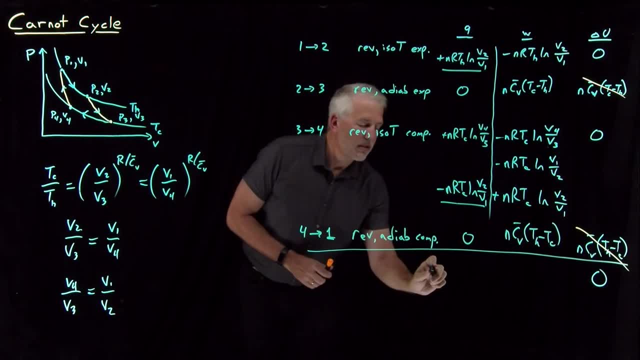 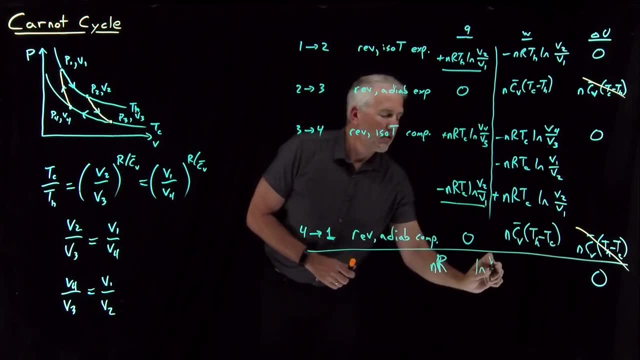 of writing this one. The total amount of heat that's associated with this process is NR. There's a log V2 over V1 that both these terms have in common. This one has a positive TH, This one has a negative TC, So I've got T hot minus T cold. 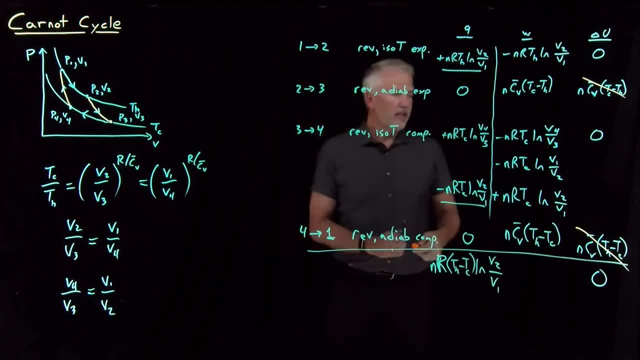 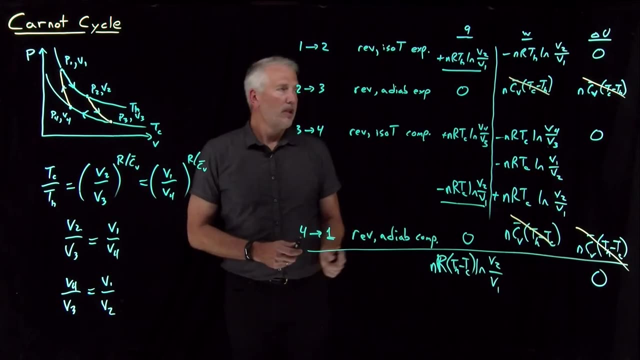 If I think about the work, there is some cancellation that happens. So NCV T cold minus T hot cancels with NCV T hot minus T cold. So that work associated with the second step and the fourth step cancel Again. remember, I only need one of these. If I look at this one and this one. 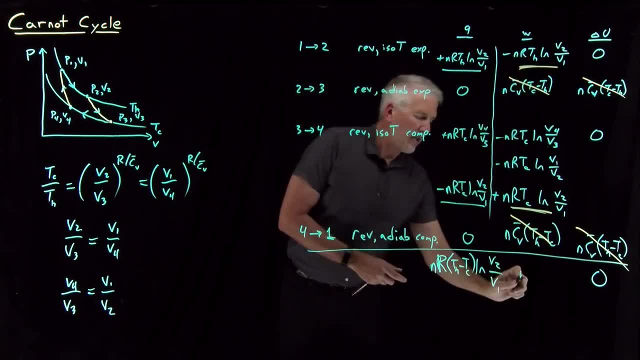 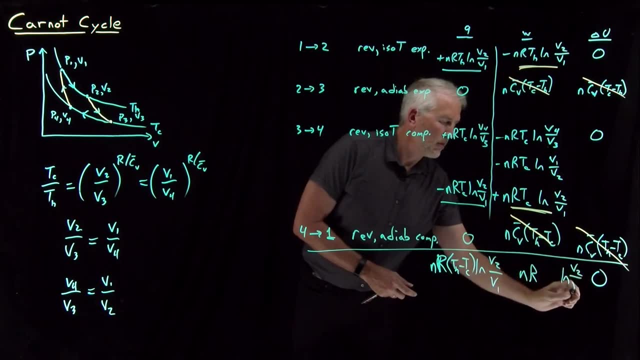 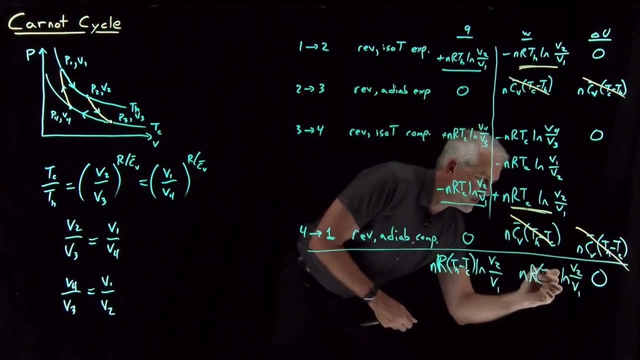 the total amount of work is. I've got an N and an R and a log V2 over V1.. This term has a minus TH. This term has a positive TC, So I'll write this one as T cold. This term has a minus TH, So I'll write this one as T cold minus T hot. 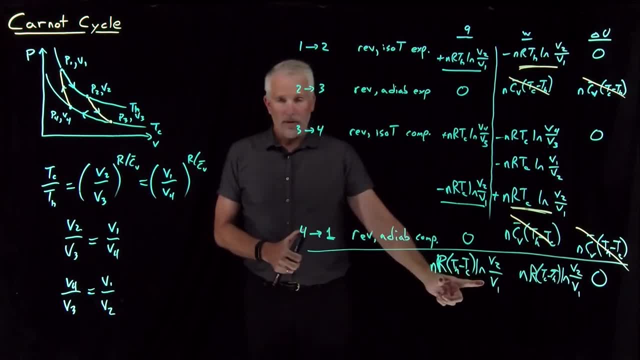 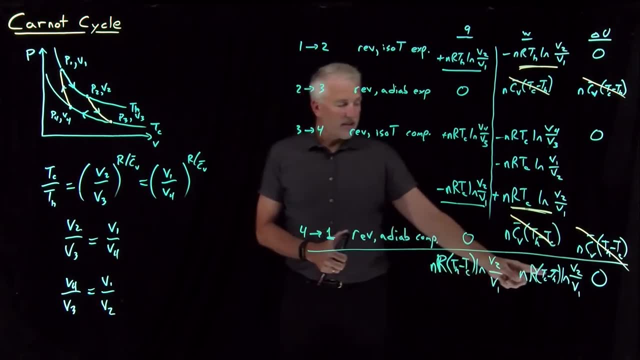 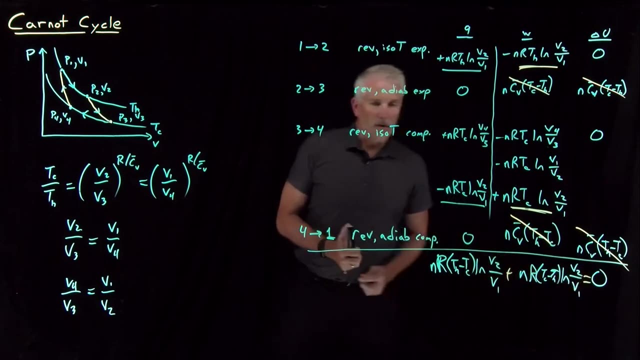 Again. not surprisingly, if I add up the heat and the work NR log, V2 over V1 times TH minus TC, add that to the same thing with a TC minus TH. those two terms cancel. So this plus this is equal to zero. Q plus W must be equal to delta U. That's still true. 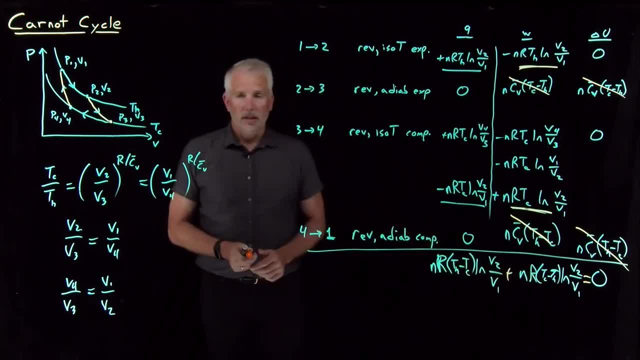 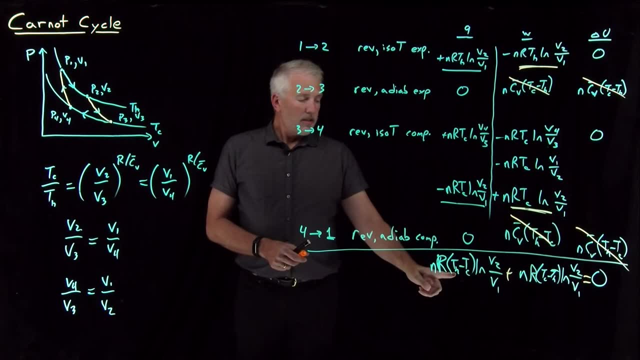 The heat is the negative of the work and vice versa. If we think about the signs of these two results, the heat- T hot- is bigger than T cold. Hot temperature is larger than the cold temperature. So this term in parentheses is positive.